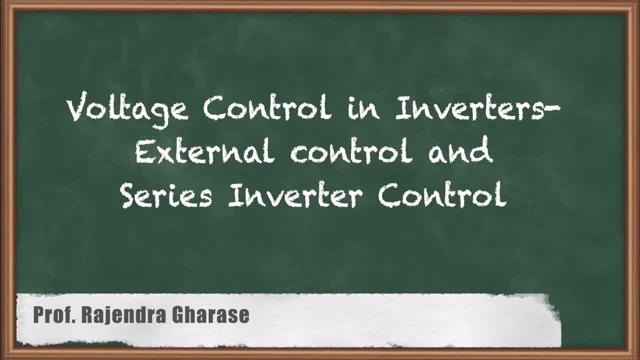 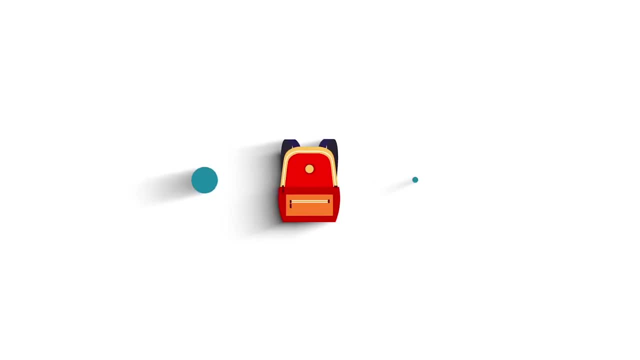 hello friends, in this video we are going to discuss the numerical related to performance parameters of inverters. okay, so let us see the example. hello friends, in this video we are going to discuss the voltage control in inverters. okay, so let us first discuss why the voltage control is required. okay, so if you check in inverter, the output is AC voltage and it depends upon its input DC voltage. okay, so if the load demands for the fixed AC voltage, the inverter must provide it, even though there are variations in the input DC voltage. okay, so here voltage control is essential to compensate the variations in input DC. 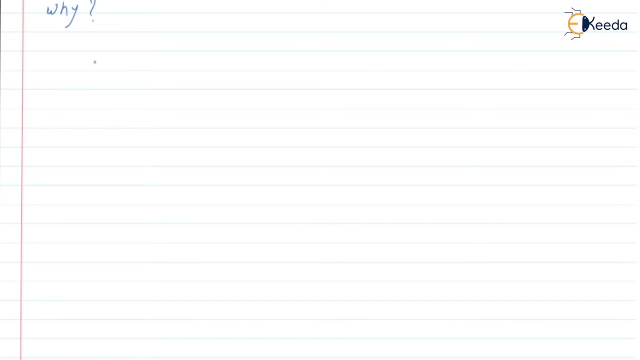 voltage. okay. also, suppose if the inverter is supplying to the induction motor. as you know, in the induction motor, where I am using the inverter, I am using the AC voltage. so if the inverter is having the very famous method of speed control, that is, the VF ratio control, okay, 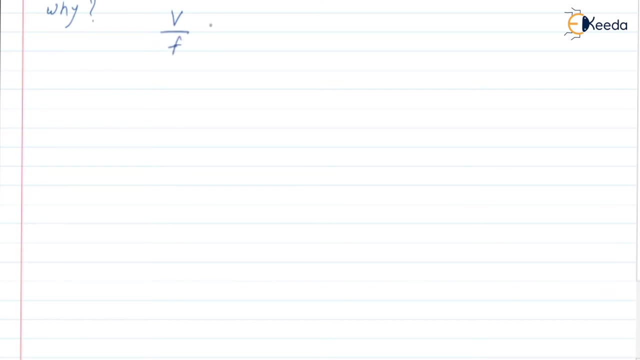 in the VF ratio control. here we need to vary the voltage and the frequency in such a way that this ratio should be maintained a constant. okay, so here, in order to vary the output voltage of the inverter and the output frequency of the inverter. right, so therefore the voltage control is required. okay, so now let us. 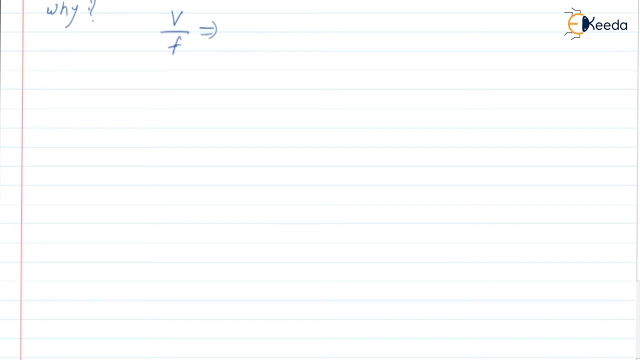 discuss the voltage control methods. okay, so in the voltage control we are having the different methods, right. so, methods of voltage control, methods of voltage control in the inverter, we are having external control, external control. in the external control, again, we are having externally controlling the AC output voltage. 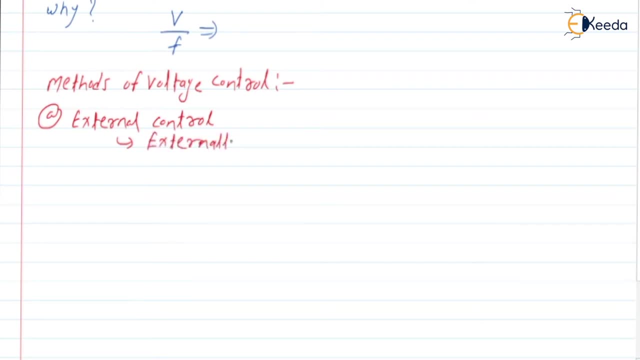 externally controlling AC output voltage, X e output voltage, and also a secondly, externally controlling DC input voltage, DC input voltage: okay, so in vision, the external control, the control is outside the inverter circuit directly to. so this is the control operation of the DC input in the inverter right and this is 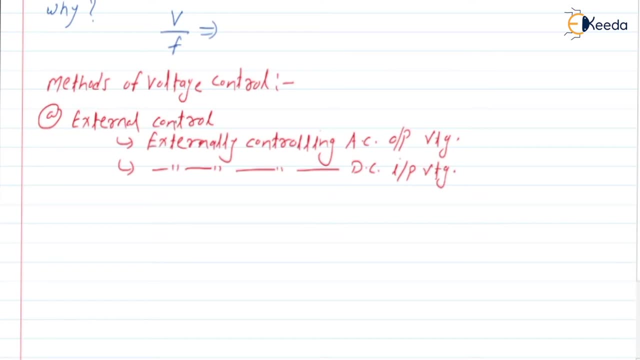 circuitry. okay. in the external control, the control is outside the inverter circuitry. okay, so in the inverter circuitry, as you know, the inverter is a circuitry where input is dc. suppose this is the inverter. input is dc, right, and output is ac. okay, so here. 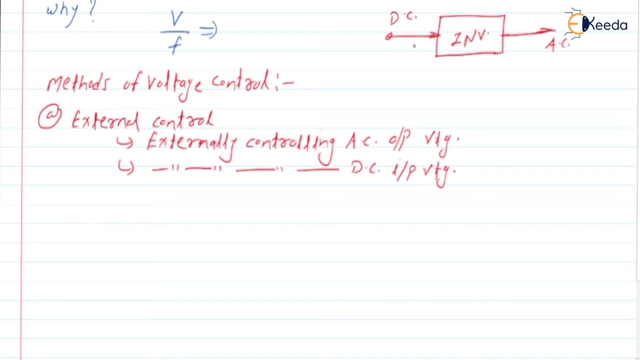 in order to control the voltage. yes, we can add the some additional circuitry or the blocks at the dc side, or we can add the blocks at the output side, that is, the ac side. okay, so accordingly, externally controlling the ac output voltage or externally controlling the dc input voltage, okay. 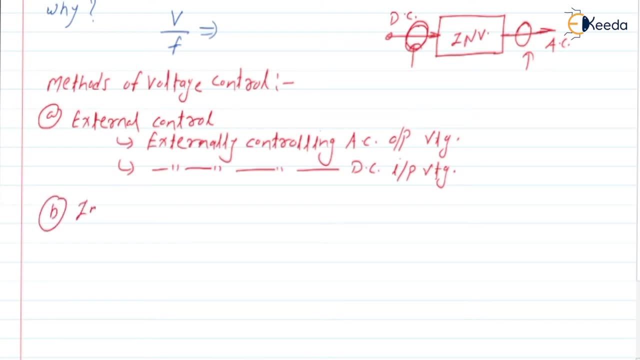 next second control is the internal control. second control is the internal control. right, internal control in the internal control. yes, the control is within the inverter itself and the control is within the inverter itself. okay, so within the inverter itself means here we are going to discuss. 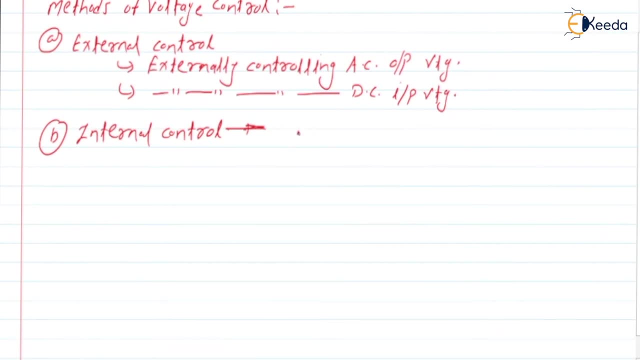 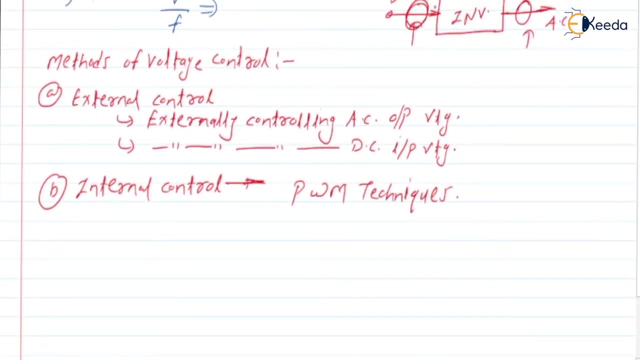 pulse width modulation techniques: okay. so pwm techniques, pwm techniques: okay. so means in the internal control we are not going to add the external blocks, okay, whereas in the external control, yes, we will be adding the external blocks. right, that's the external circuitry right, either to the input side or to the output side of the inverter, okay. 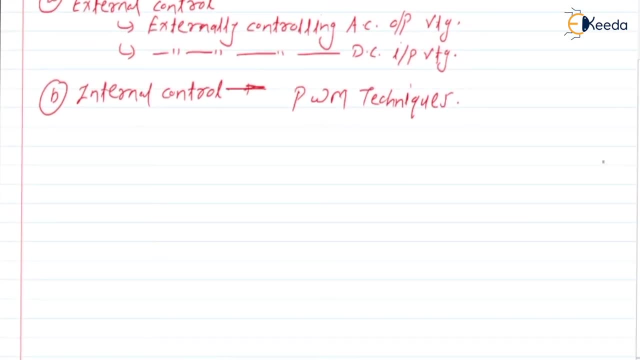 so let us first discuss the external: externally controlling the ac output voltage right, externally controlling the ac output voltage serviced. so first externally controlling ac output voltage, ac output. okay, so here means, at the output side right we are going to vary the inverter output by adding the additional. 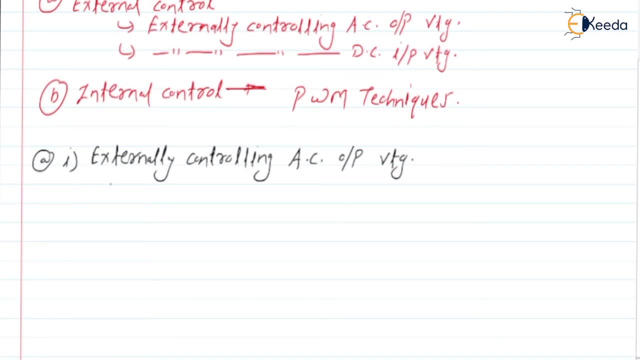 blocks by adding the external blocks. okay, so we can vary it either by AC voltage control, by adding the AC voltage controller block at the output side of the inverter. second is series inverter control. we can use the series inverter control, series inverter control- okay, so in this way we can vary the output voltage okay. 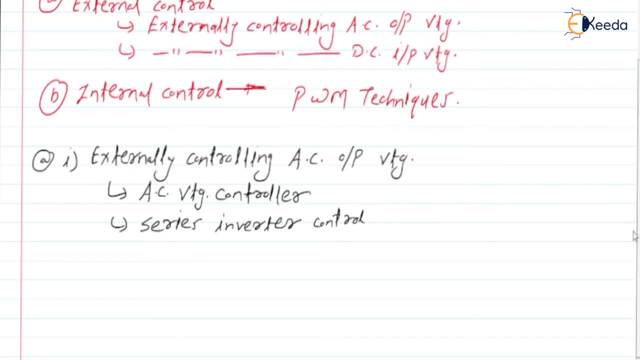 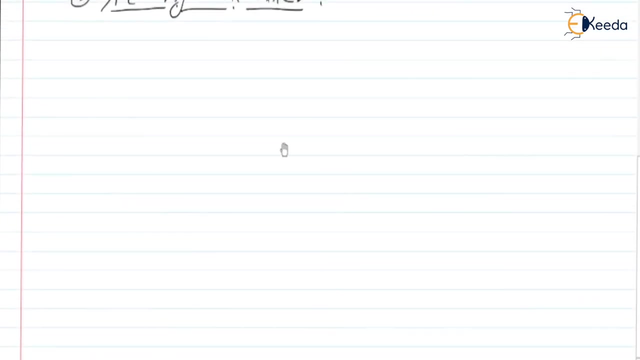 so let us first discuss AC voltage control, right, AC voltage control. so in that AC voltage control or controller, so in this method of controlling the inverters output voltage. okay, so what we are going to do is we are going to add, we are going to add external block, right, we are going to. 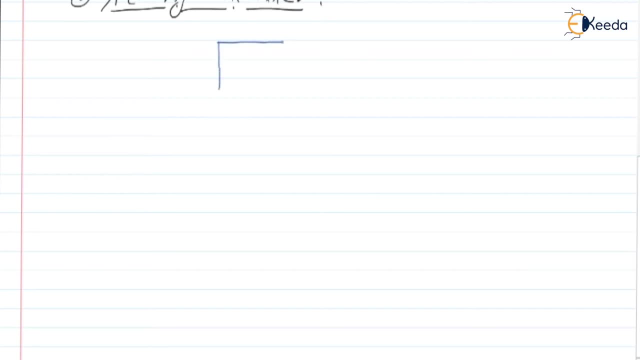 add the external block, that is, the AC voltage controller, right at the output side of the inverter. okay, so here you have the inverter right. next here we have the constant DC voltage. constant DC voltage right and any is output of the inverter is given as an input to the ac voltage controller right ac voltage controller. 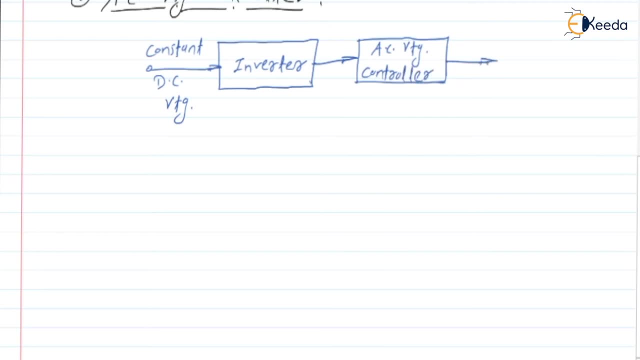 the ac voltage controller is the block which converts the fixed ac to the variable ac. okay, and that controlled ac is given as an output or as an input to the load, right? so if you check here, yes, here we are having the fixed ac output of the inverter and here we will be getting the 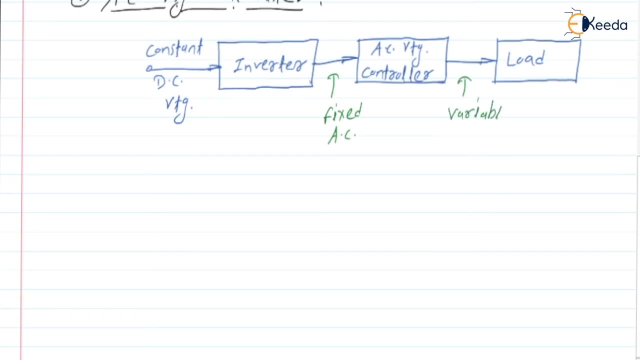 variable ac or the controlled ac. variable r- controlled ac. variable r- controlled ac- right, are you getting the point? okay, so here we are adding the ac voltage controller at the output side of the inverter right. next second meter, let us discuss, yes, the second one right in the external control right, or the ac hold externally controlling the. 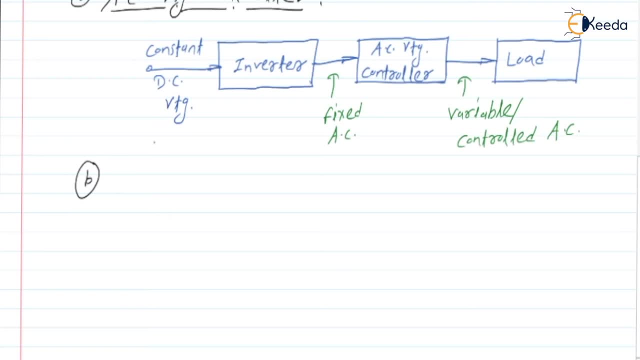 ac output voltage right in that it is a series inverter control right. series inverter control, series inverter control in the series inverter control. yes, we are going to use the output voltages of the two inverters right, and we are going to connect them in series with the help of transformers. okay, with the help of transformer. so here, 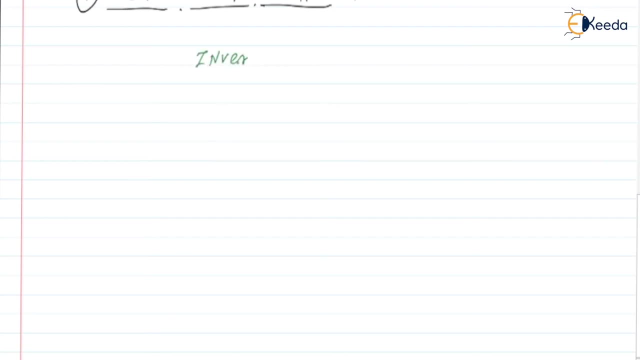 will be having the inverter one. yes, we are having inverter one and the second inverter. okay, Input to both the inverters is same constant DC voltage is a constant DC voltage, right? Next, output of the inverter one is connected to the primary winding of the first transformer. 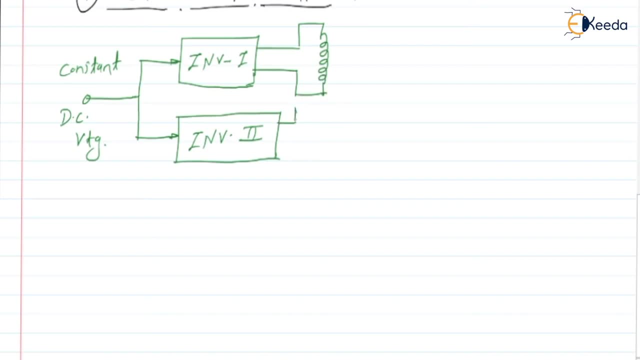 and the output of the second inverter is connected to the primary winding of the second transformer. okay, So in this way we have connected. Next, the secondary windings of both the transformers are connected in such a way that, whatever the industrial voltages, will be there in the secondary windings, right. 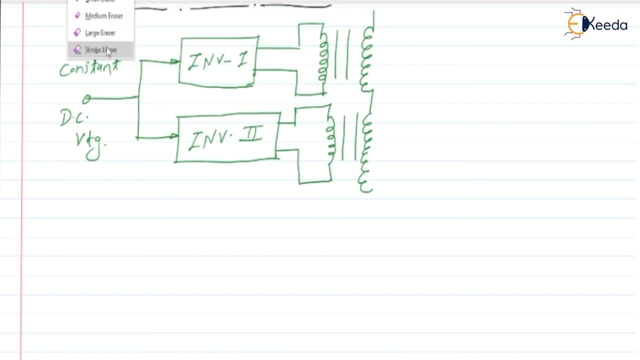 Whatever the industrial voltages will be there in the secondary windings- right, Those will be additive, right Those will be additive And having a load. This voltage is VL, here it is a V1,, here it is a V2, right. 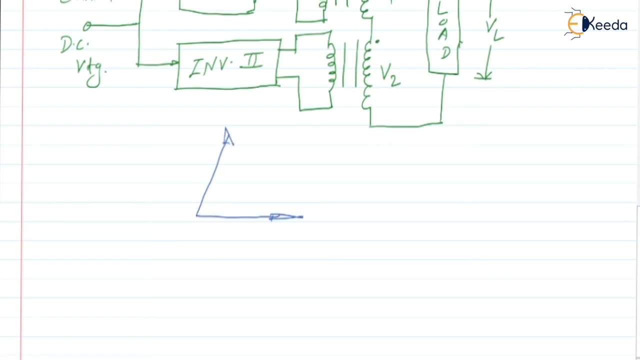 So here we will be getting the output voltages. we will be getting the output voltages of both the inverters. right, those are not in phase, okay, so it is like this. so this is the V1 we are having. here it is a V2 we are having. okay, so here it is a V2.. 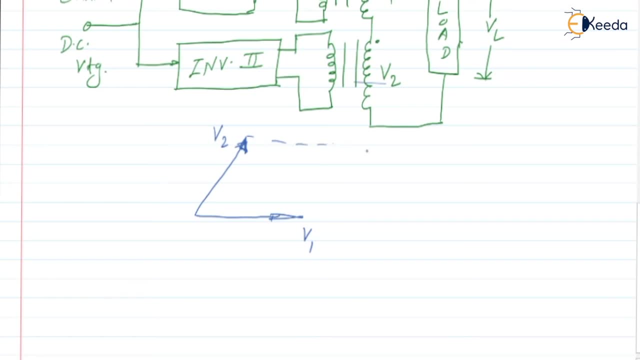 Right, and the addition of the two is equal to. so this will be your VL, that is the load voltage. okay, so this angle is theta. what is VL? VL is equal to. according to law of parallelogram, VL is equal to under root. yes, V1 square. 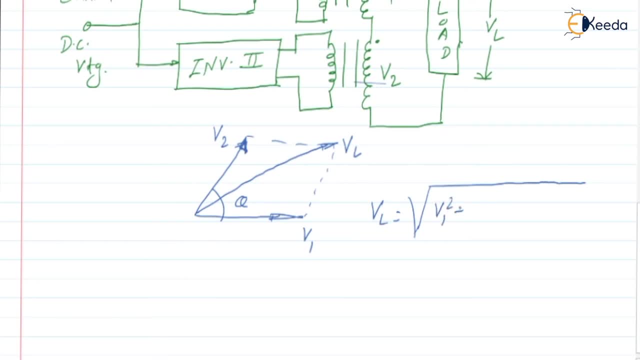 V2.. As V2 square, V1 square plus V2, square plus 2 times V1, V2 into cos of theta. theta is the angle between V1 and V2, okay, so here let us discuss how it works, right, so series. 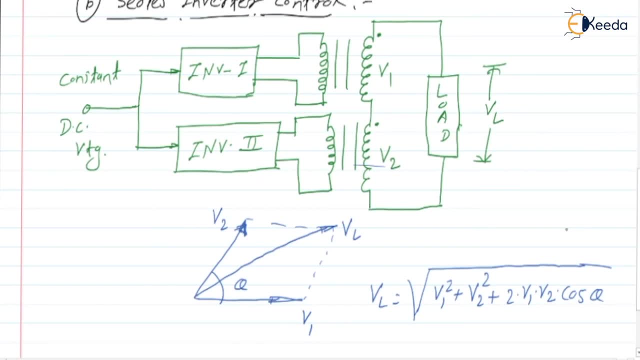 inverter control. so ultimately our task is to control the voltage across the load, right voltage across the load we need to control. okay, so for that case here we are using two inverters: inverter 1 and the inverter 2.. 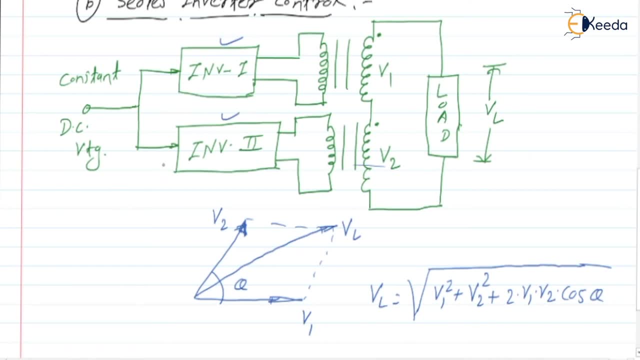 The input to both the inverters is same, that is, the constant DC voltage. okay, as we know, inverter is a circuitry which converts DC to AC, so if the DC is constant, so we will be having- yes, the output voltage is also constant. right, output voltage is also constant. 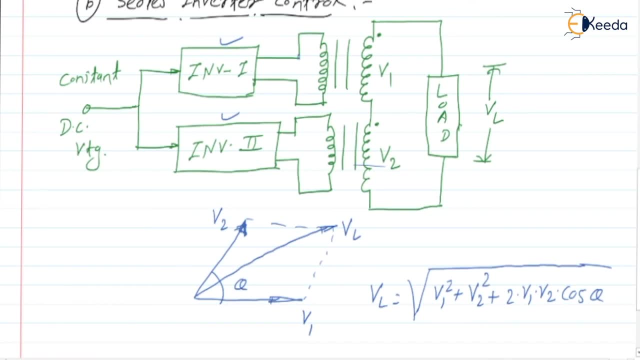 because we are not changing circuitry inside the inverter. okay, so here we will be getting the voltage right. suppose this voltage is V1 dash. suppose this voltage is V2 dash. okay, This is the primary winding of the transformer. here it is the secondary winding of the transformer. 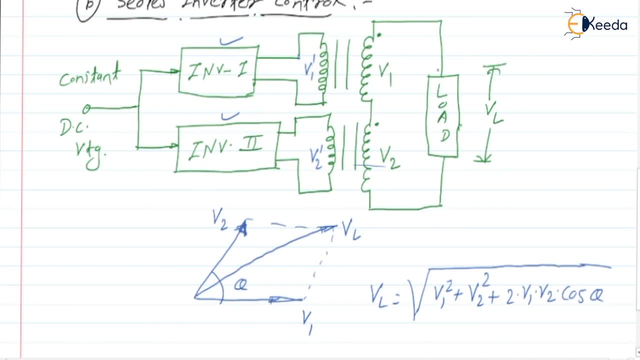 right, as well as transformer is the circuitry or machine which transfers electrical energy from one circuit to the another circuit. okay, so here EMF induced at the secondary side is V1, here it is the V2, here the secondary windings are connected in such a way that 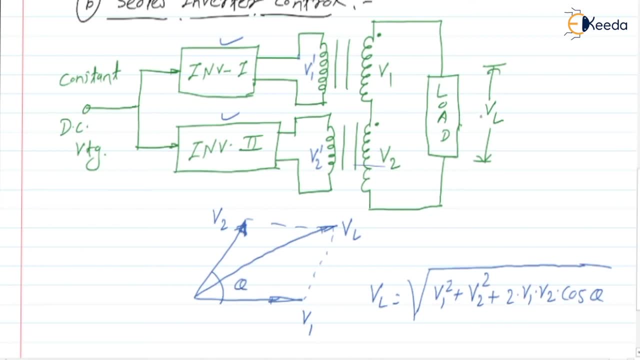 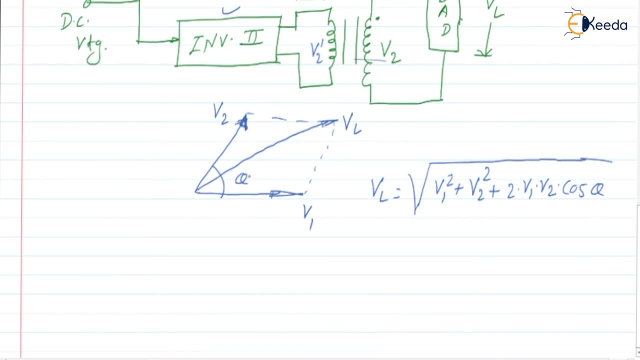 the resultant voltage will be addition of the V1 and V2, that is equal to VL. okay, Now here how to control the VL. okay, how to control the VL. here we are controlling the VL right: by Varying the phase difference between V1 and V2, by varying the phase difference between 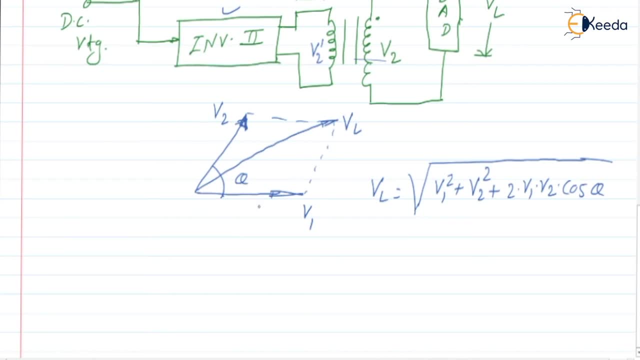 V1 and V2, okay, so if you check in this circuit, V2 is leading to V1 by angle theta, V2 is leading to V1 by angle theta. so how to get, yes, the how to create that phase difference between: 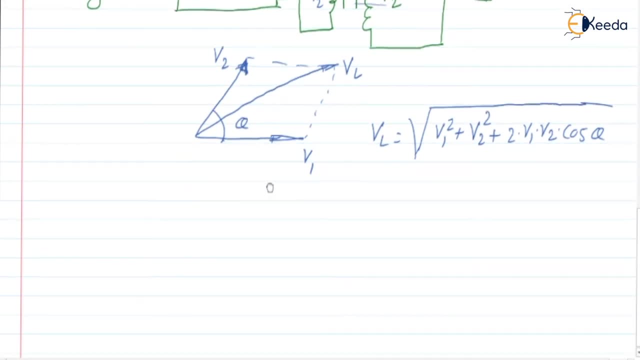 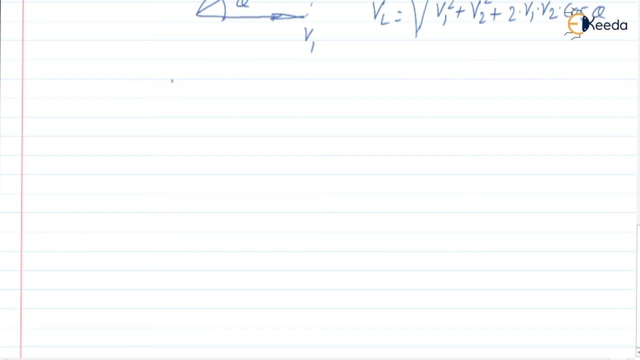 the V1 and V2,. yes, so here we need to turn on the switches right in the in the inverter 1 and inverter 2 in such a way that, yes, Suppose, If this is the waveform for V2, that is the inverter 2's output. okay, so suppose T here. 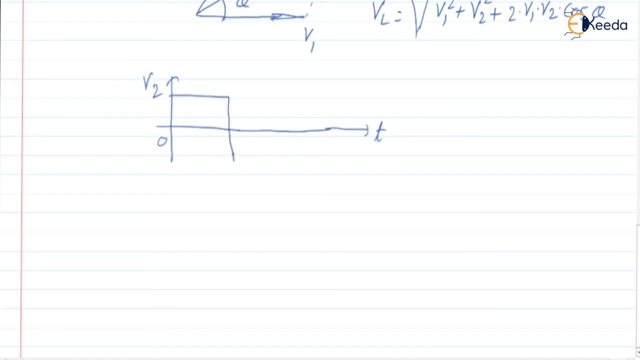 it is 0,. okay, this is the T by 2,. here it is T. here it is 3T by 2, okay, this voltage. suppose this is the full bridge inverter, Then it will be EDC. this will be minus EDC, right? this will be minus EDC, right, so here. 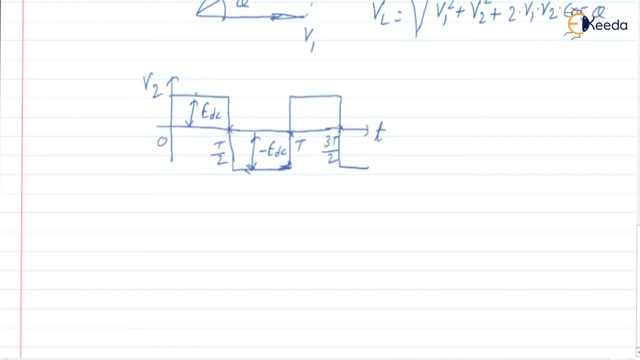 during 0 to T by 2,. yes, output voltage is EDC means switches S1, S2 will be in the on state for second inverter: From T by 2 to T. output voltage is minus. EDC means switches S3, S4 will be in the. 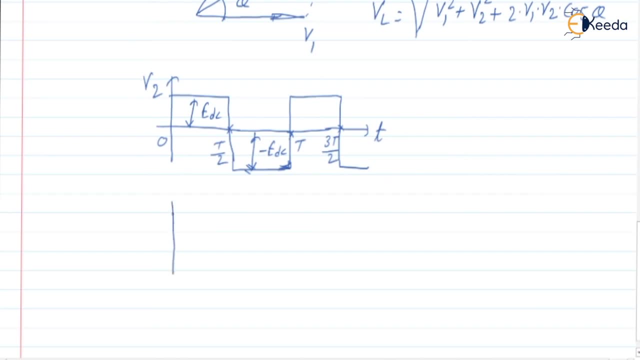 on state. okay. so, similarly, in order to create a phase difference between V1 and V2, right here we need to operate the switches of inverter A, Okay, Okay. So we need to operate the switches of inverter A or the inverter 1 in such a way that there. 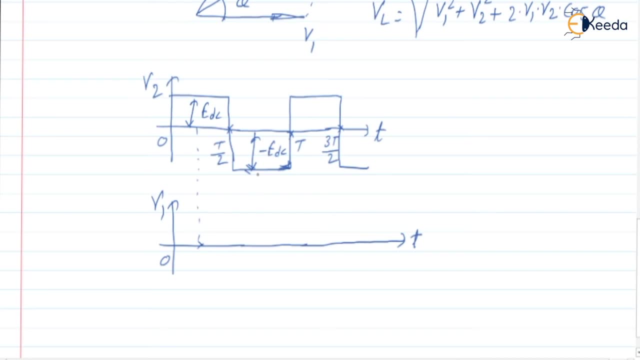 exists a phase difference of angle theta right. there exists a phase difference of angle theta between the two inverters right. So here means at this instant we are going to turn on the switches S1, S2,, right we. 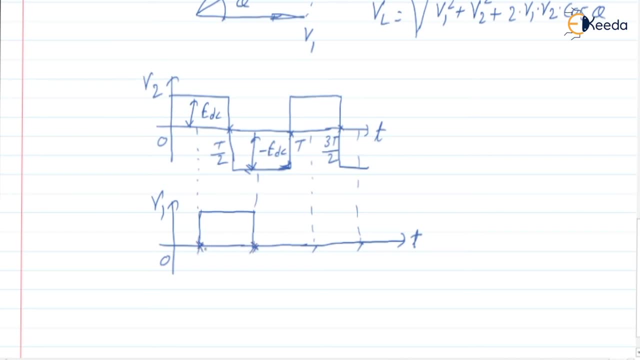 are going to turn on the switches S1, S2 of the first inverter right during this interval. okay, So here, S1, S2 turned off, S3, S4 turns on right. Similarly, here again, S1, S2 turns on, and so on. this goes on repeating, okay. 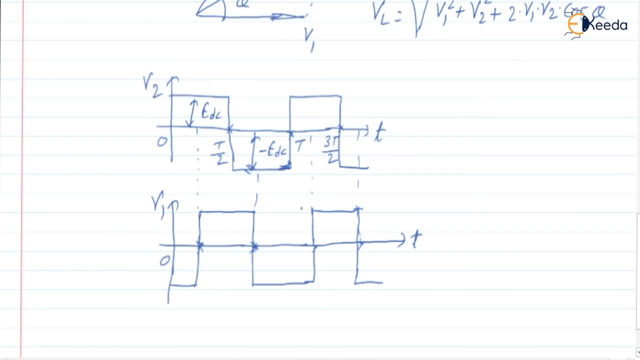 So in the continuous cycle it will be like this: What is the phase difference? Yes, this is the EDC, this is the minus EDC, right where? yes, so if you check, what is the phase difference between V1 and V2?? 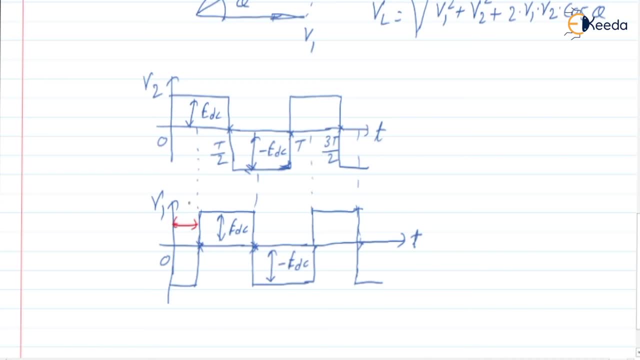 Yes, you check the phase difference. here is the angle theta right. here v2 is leading to v1 by angle theta right. so v2 has started positive edc at zero only, but here it is starting after this instant. are you getting the point? okay, so this phase difference is theta and this phase difference. 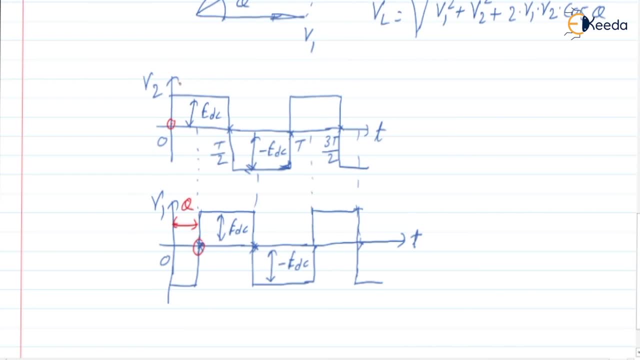 is theta. okay. so here for second inverter. we are turning on s1 s2 during these intervals. s1 s2 on and here s3 s4 on right, and again s1 s2 will be the on state right, s1 s2 on. similarly for the. 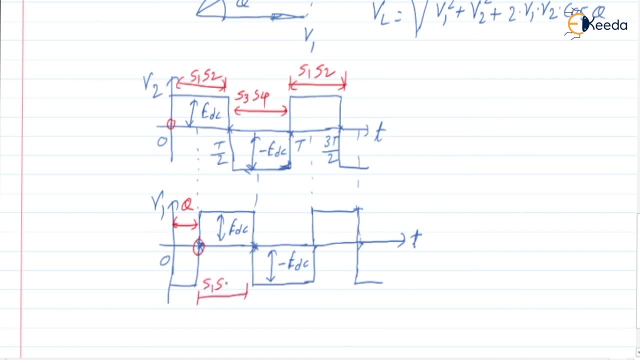 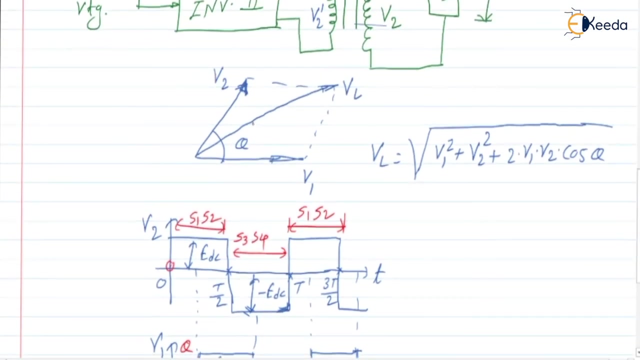 first inverter. it will be like: here we need to on s1 s2, here it is the s3 s4, right s3 s4 and so on. is this clear? so, accordingly, we can create any phase difference between v1 and v2. okay, and by varying the phase difference between v1 and v2, yes, we can control. 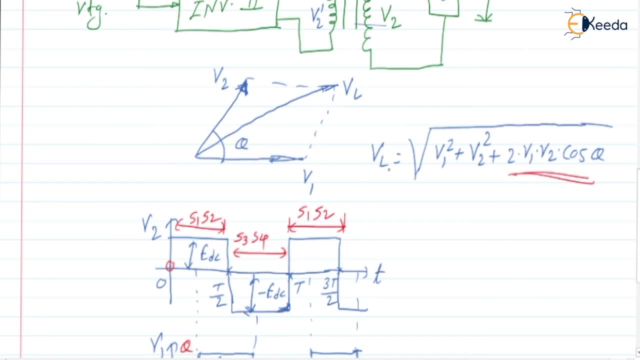 we can control the load voltage across the load. okay, so this is the one way of controlling the voltage of the inverter. okay, at the output side. at the output side. next, externally controlling the dc input voltage. externally controlling the dc input voltage: okay, so now how to control. 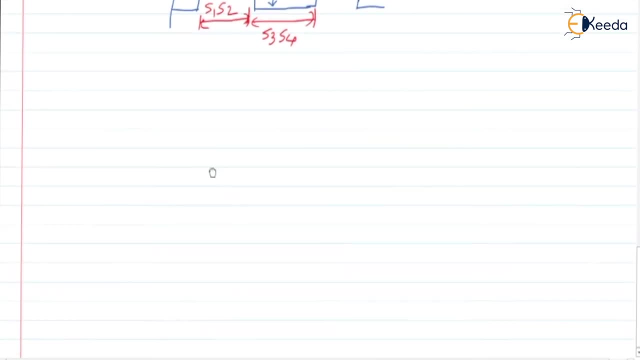 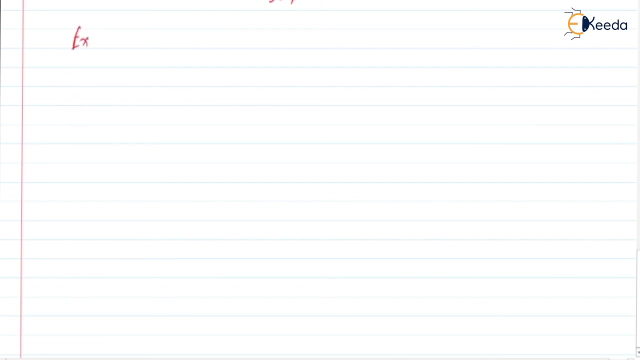 or how we can control the dc input voltage of the inverter that we are going to discuss now. okay, so, externally controlling, externally controlling dc input voltage, dc input voltage: okay now. so now, just like a in the externally controlling the ac output voltage where, yes, we added a ac voltage controller. 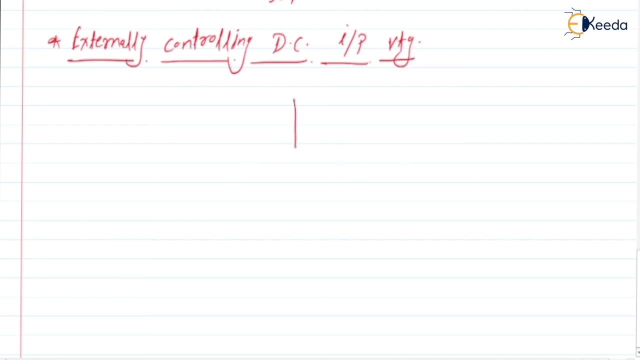 block right. so so now here we are going to add external blocks at the input side of the inverter. okay, so suppose here, wearing the inverter right, output of the inverter is given to the load right. ultimately, our task is to vary the voltage across the load right, to vary the voltage across 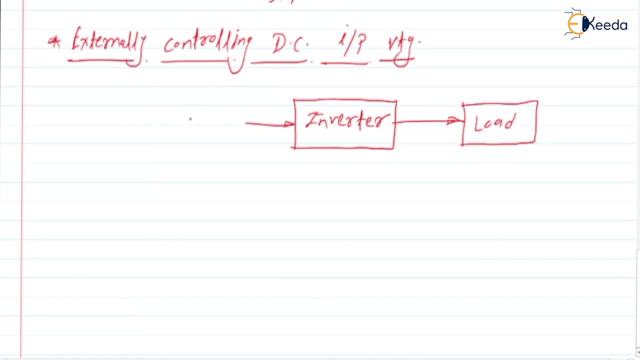 the load right next. so here we can use the rectifier, rectifier circuitry. this is not the unique circuit, again, right? so suppose the input, wherever the ac voltage. if input is ac voltage, it is given to the rectifier. rectifier gives an output as an. 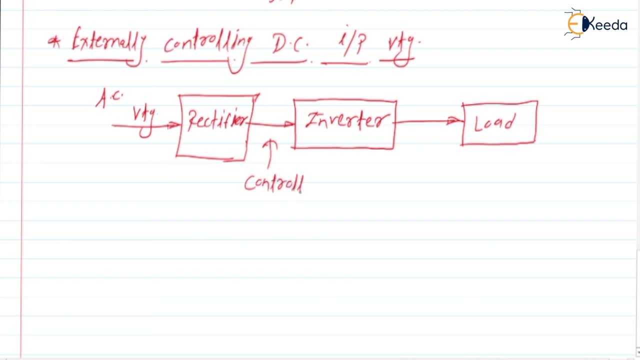 controlled dc means variable dc. if that control dc is given as an input to the inverter, yes, inverter will give the output as a controlled ac, controlled ac and that controlled ac, yes, it can be given to the load right and due to that you can control the load voltage right load voltage. this is the one way. 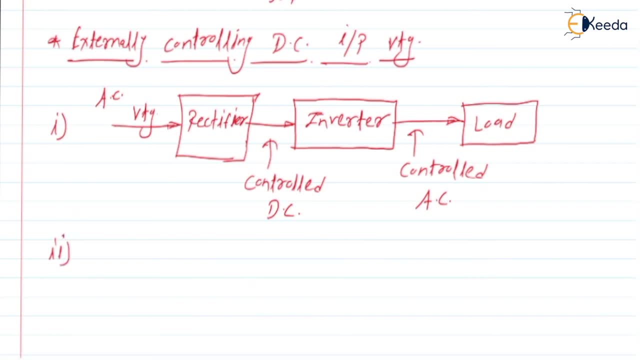 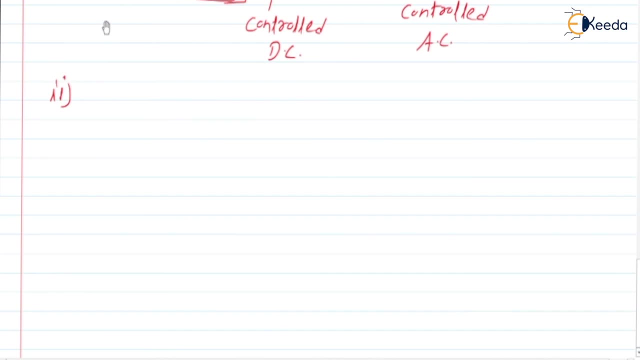 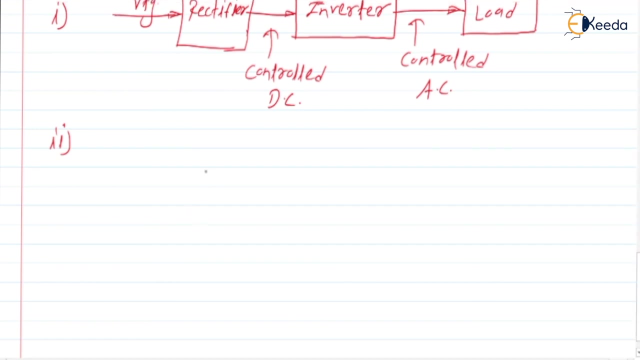 the second approach is: yes, we can add. the second approach is: yes, we can add this. suppose this, suppose this. suppose we are having dc voltage as an input, right dc voltage as an input, and we can add the copper block here. copper is the circuitry which converts extra dc to variable dc. okay, so this is here we are having. 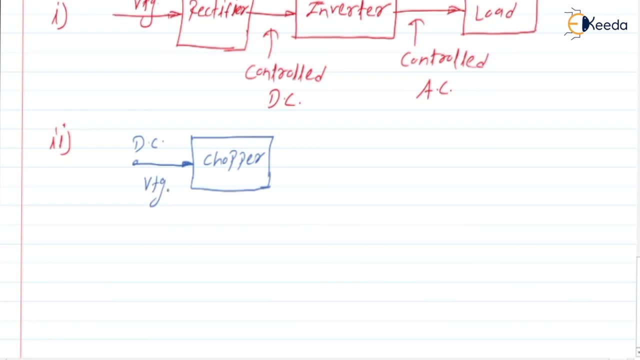 the dc voltage, which is the input to the chopper. next output of the chopper is: it is a variable dc, right? it is given to the rectifier. sorry, it is given to the inverter. we can give it to the inverter directly, right, because input to the inverter is dc. okay, so here we will be having controlled dc. 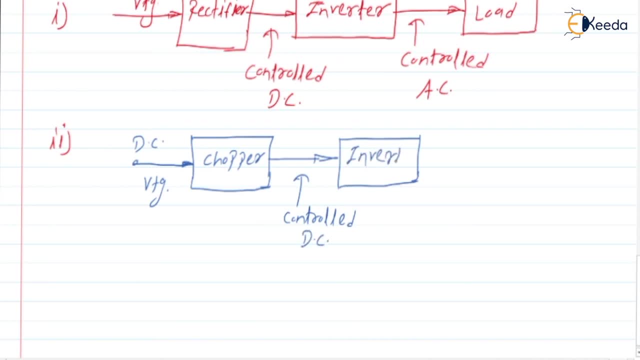 next, that control dc is given as an input to the inverter and the inverter if the input to the inverter is changing. so whatever the output is, we will be getting the controlled ac, controlled ac, and that controlled ac can be given to the load right can be given to the 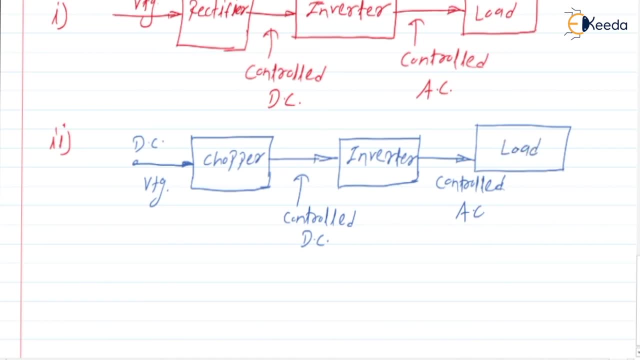 load. okay, and accordingly, yes, we can vary the load voltage. okay, this is the second example, right? so these are not the only ways. okay, we can add: yes, suppose the input voltage is ac, if it is given to the ac voltage controller, after that it is given to the rectifier and then we can give it to the 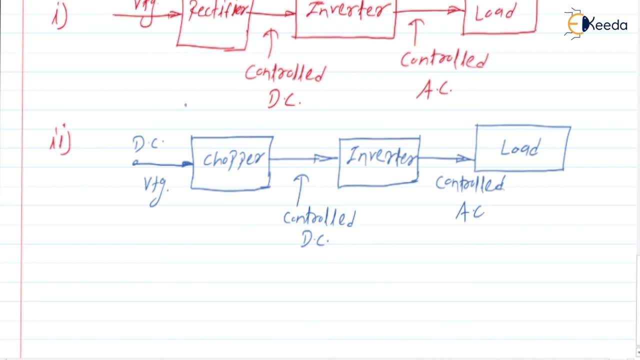 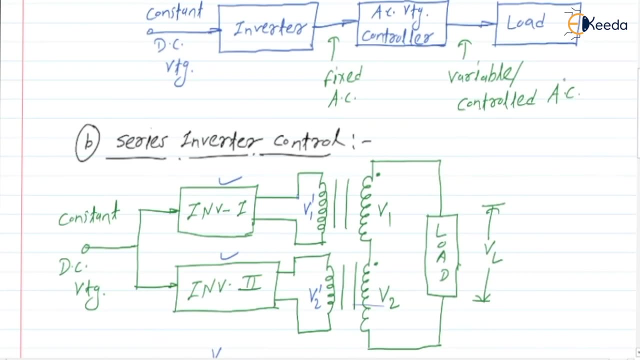 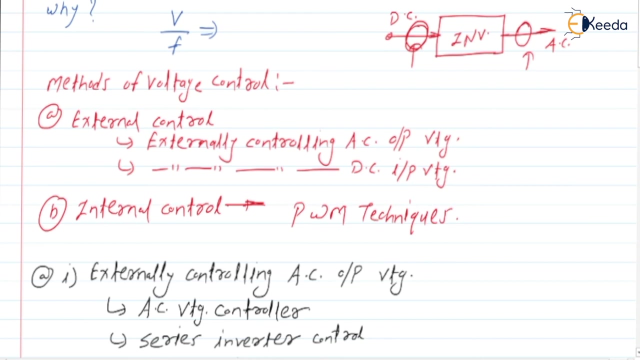 inverter also. okay, so we can add number of blocks at the input side. okay, so this is about the voltage control in the inverter thread. but by externally controlling the voltage i'm saying okay, in the next video we'll discuss the internal control. thank you you.